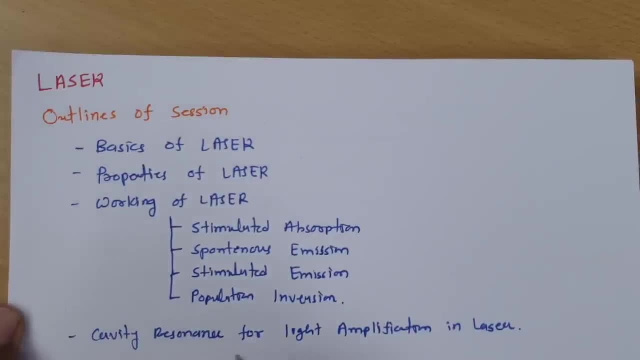 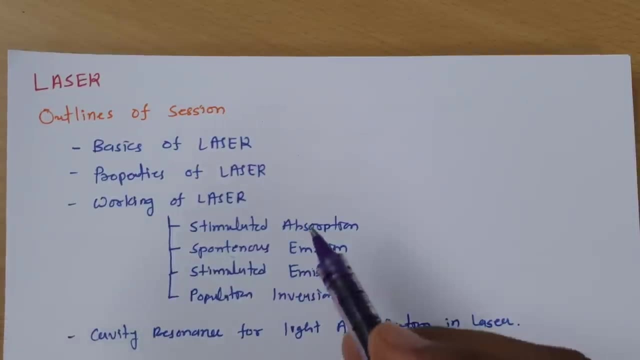 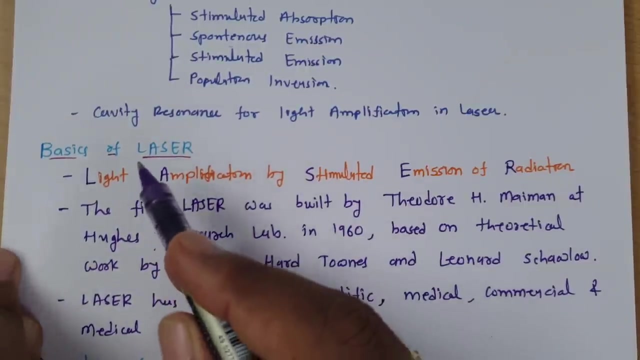 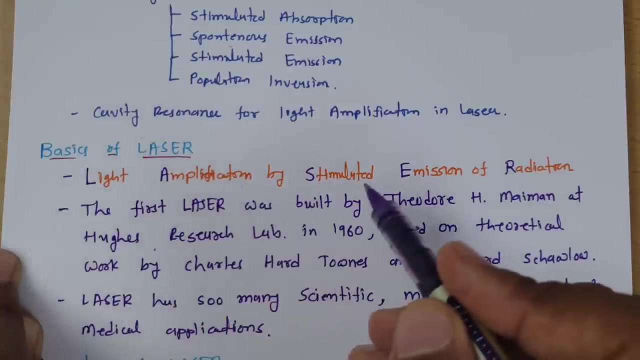 And then with the study of cavity resonance for light amplification in laser, I'll conclude this session. So let us begin this session with first agenda, that is, basics of laser. Now see first of all what is the full form of laser, So LASER, and that full form is light amplification by stimulated emission of radiation. 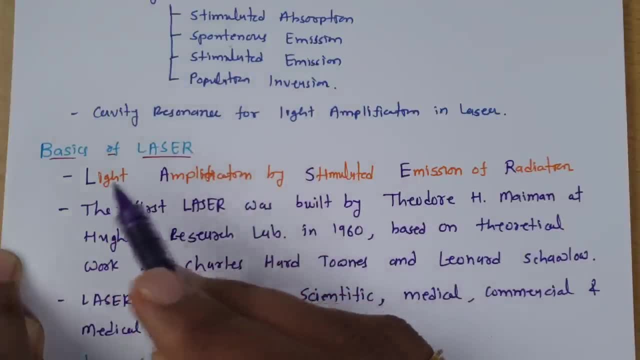 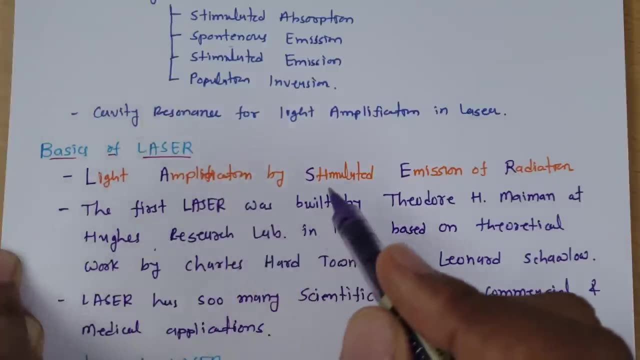 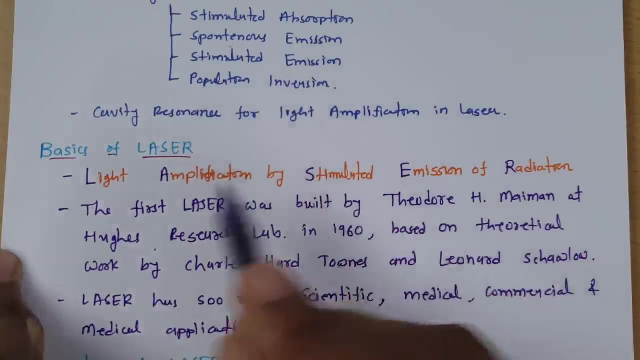 So here, based on this, LASER- in short it is referred as laser- which is light amplification by stimulated emission of radiation. So as per this full form, one can clearly see it is what light amplification, and that is by stimulated emission of radiation. So all those terms that I'll be explaining in further part of this session. 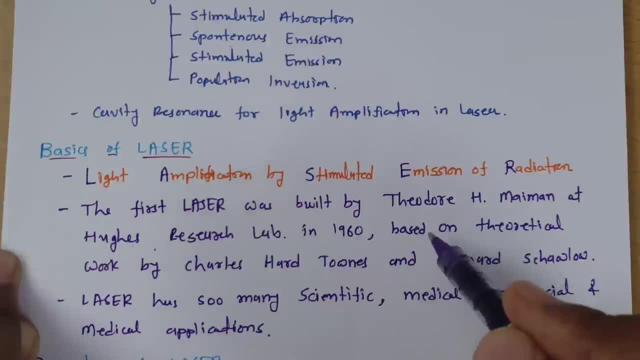 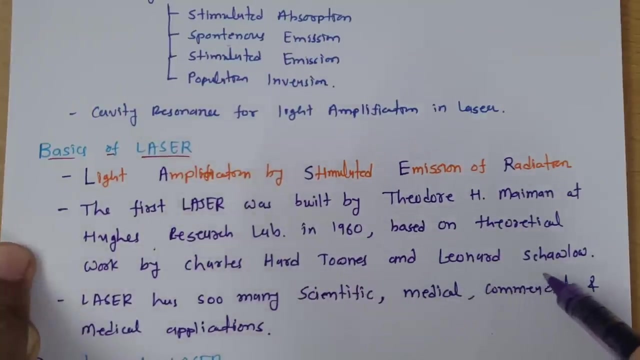 See laser was felt, first build up by Theodore H Maiman at UGIS Research Laboratory in 1960, and that was based on theoretical work done by Charles Hard Tonans and Leonard Scolop. So that was first built up by Theodore H Maiman at UGIS Research Laboratory in 1960. 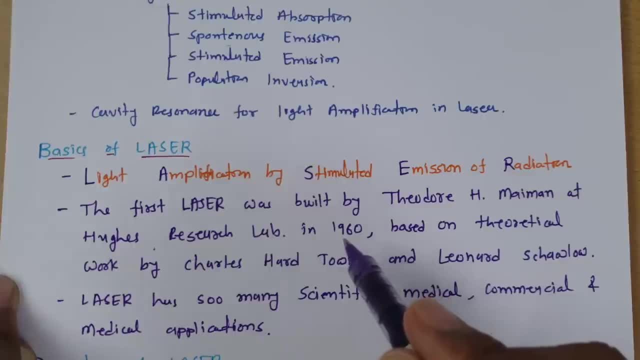 and working phenomenon that is similar to MASER microwave amplification by stimulated emission of radiation. So that was built up in 1954 and then, after this, laser have built up, that is for light amplification of stimulated emission of radiation, and laser is having so many applications like 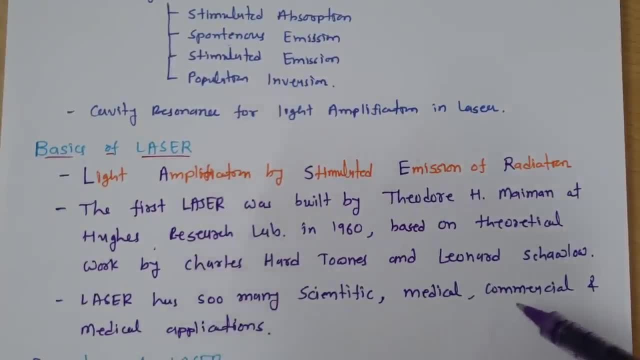 scientific applications, Medical applications, commercial applications, as well as medical applications and military applications even there. So there are so many applications which is there with laser. that's why this device- that is what so useful in communication, as well as in some basic commercial applications. 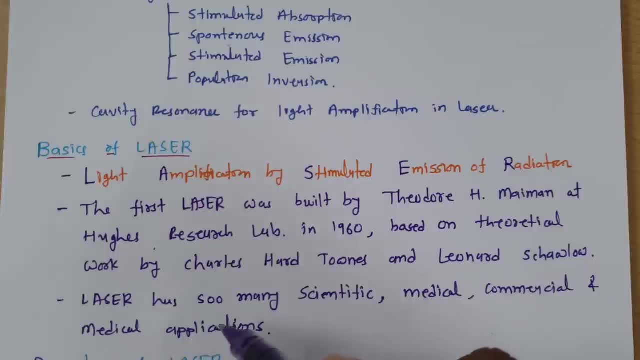 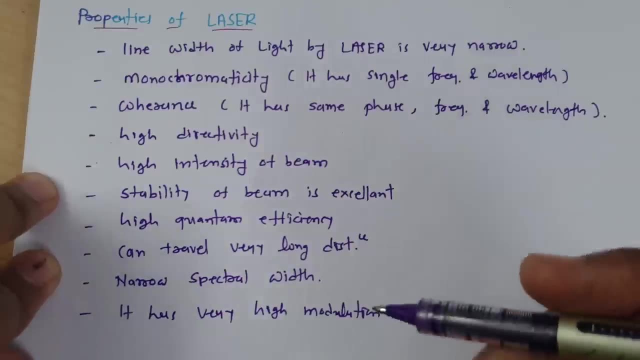 So let us try to understand why there is that many applications. So let us try to understand what kinds of applications are there with this laser. So for that, first I will explain you properties of laser and then we will go for how laser is working. 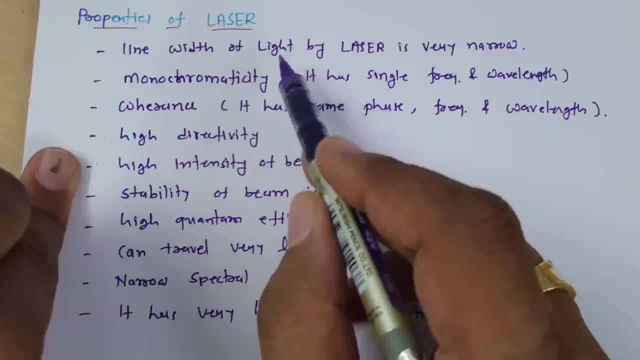 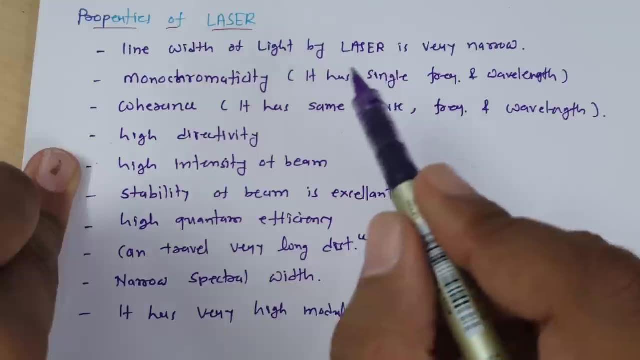 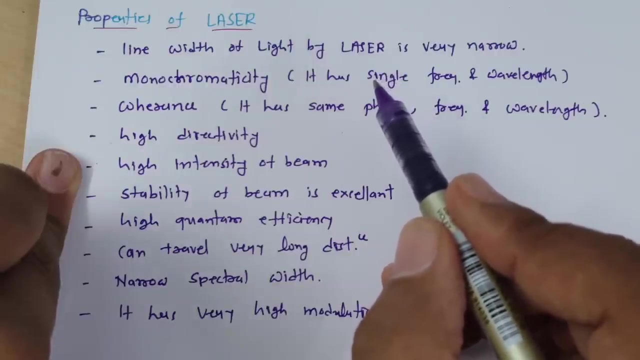 Now see first property, that is, line width of light by laser is very narrow. so when you have any laser, line width of that is very narrow. I think all might have seen laser. it's line width is very narrow. that's why you can have sport and that is why the laser is very narrow. 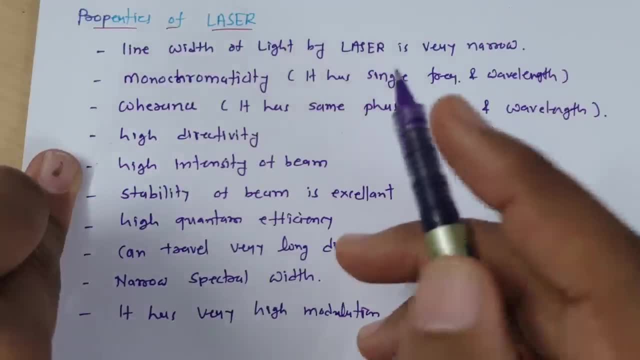 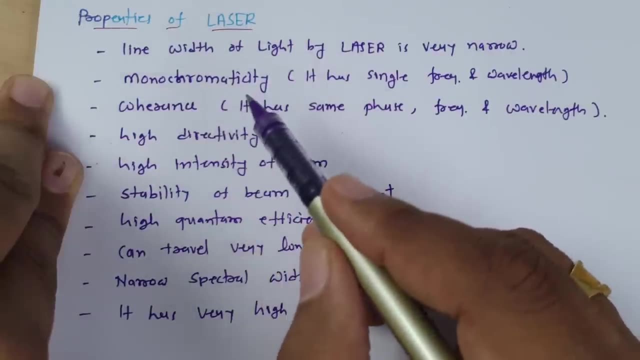 I am going to explain the properties of laser and then I will go for how laser is working, which you can transmit it to very long distance, so that sport has been created. because of line width is very narrow, monochromaticity is there with laser. 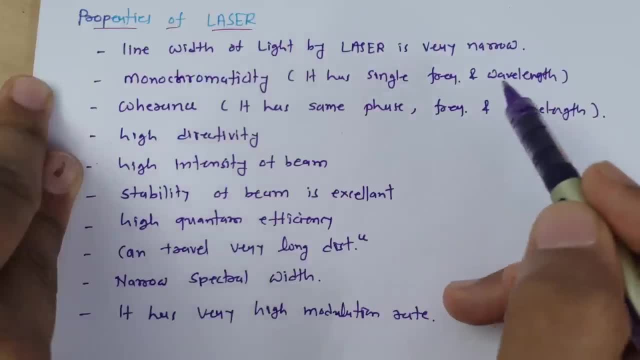 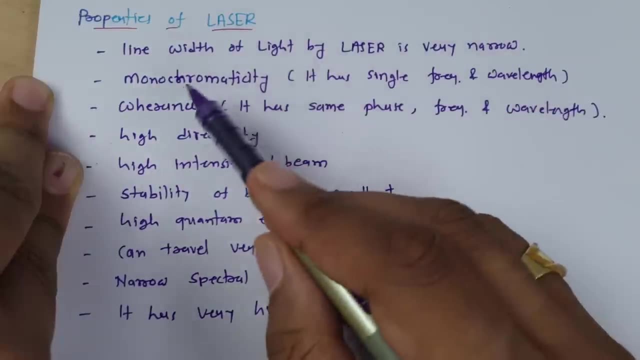 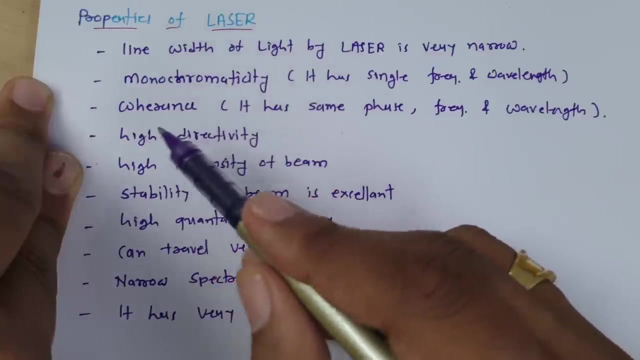 monochromaticity means it has single frequency and wavelength. so when you work with laser it is having single frequency and wavelength, so it follows monochromaticity. there is coherence light generated by laser. so coherence light means it has same phase and frequency, or one can say same phase and 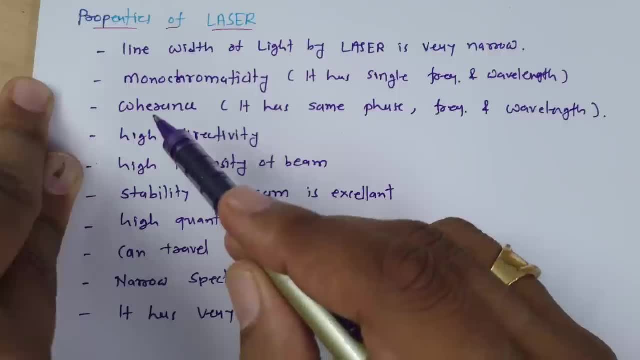 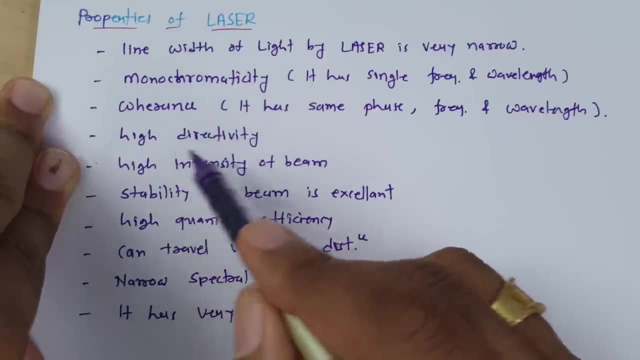 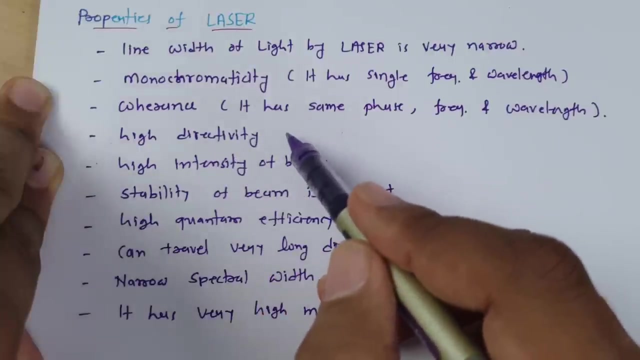 wavelength which is there with laser. so light transmitted by laser is coherence light. it is having very high directivity, so directivity is very high. that's why we can send this signal of light to very long distance by using laser. high intensity of beam can be generated by laser. 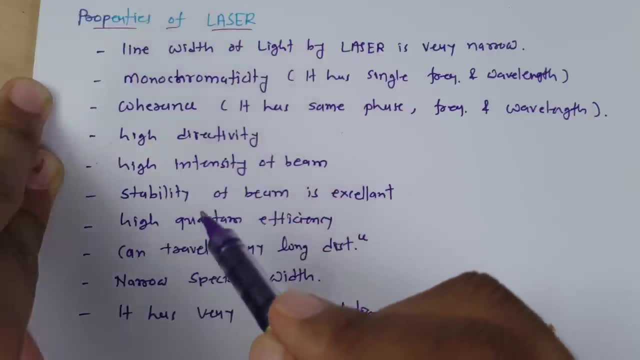 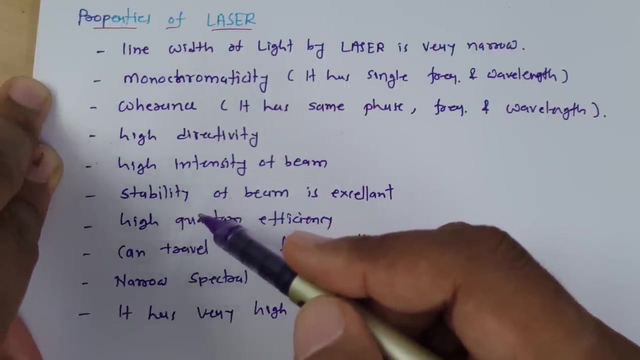 stability of beam can be generated by laser. stability of beam can be generated by laser. stability of beam is excellent by using laser. compared to LED. stability of beam is very stable in case of laser. so for long distance transmission in optical fiber communication we use laser rather to go for LED. so we go for laser for. 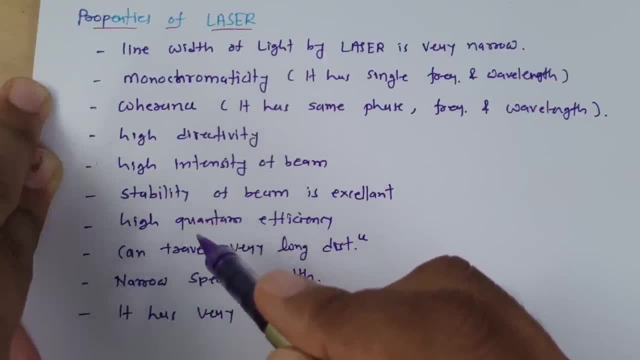 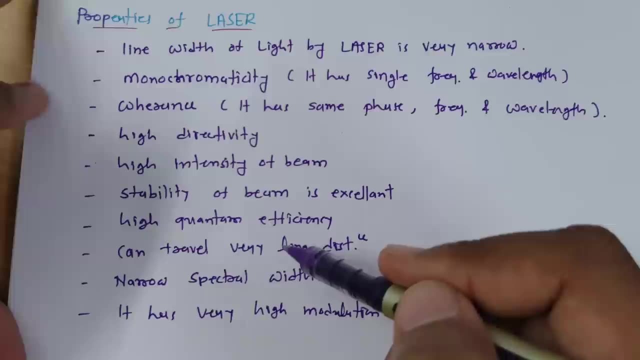 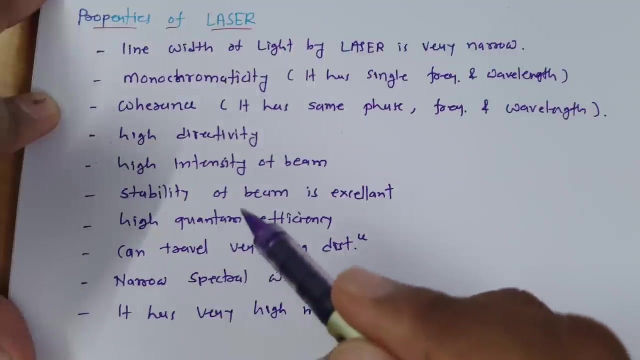 long-distance transmission of signal in optical fiber communication. it is having high quantum efficiency and quantum efficiency is way better than LED. in case of laser, it can travel to very longer distance because of directivity is very high. when you work with laser you will be finding spectral width is very narrow. so for laser spectral width is very narrow. why? 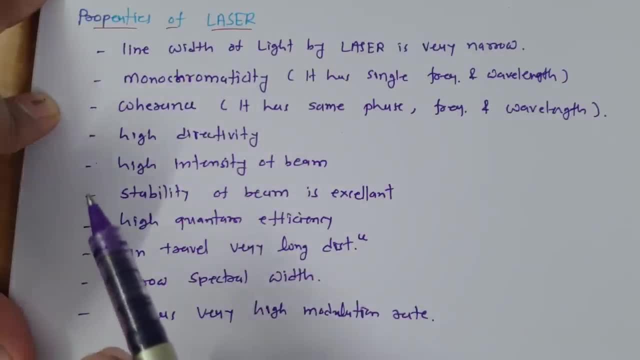 the reason is it follows monochromaticity, so it is having single wavelength or frequency, so spectral width is very narrow. it is having very high modulation rate, so modulation rate of signal will be very high, so we can have higher data rate of transmission by using laser. so these are the important properties which is there with laser and how. 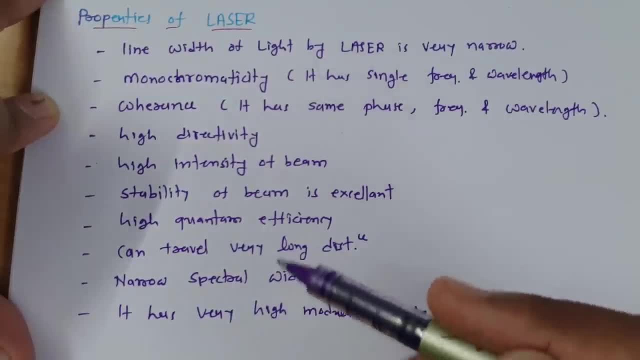 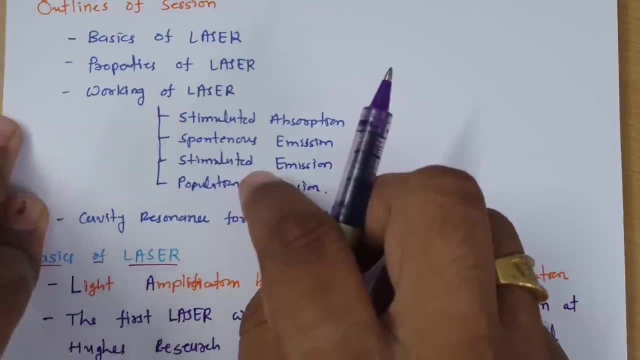 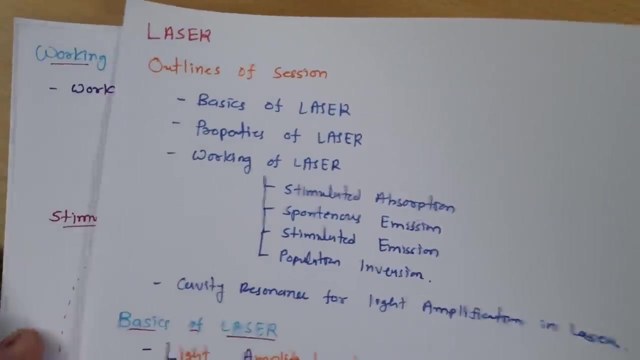 those properties are getting achieved. for that we need to understand what is the working of laser and, as i have told you, initially working is been subdivided into four parts, so i'll explain all four parts one by one, so one can easily understand how laser is functioning. now see. 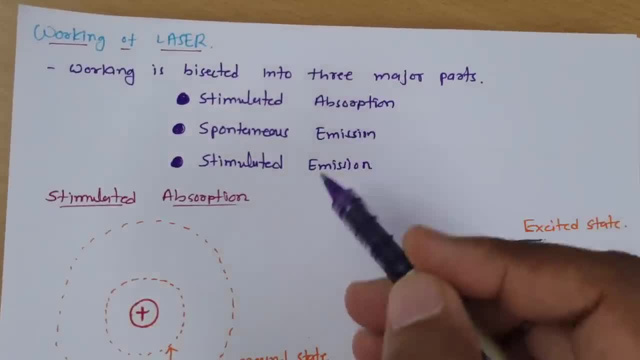 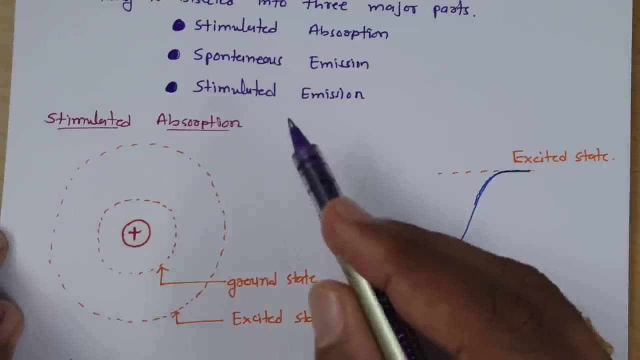 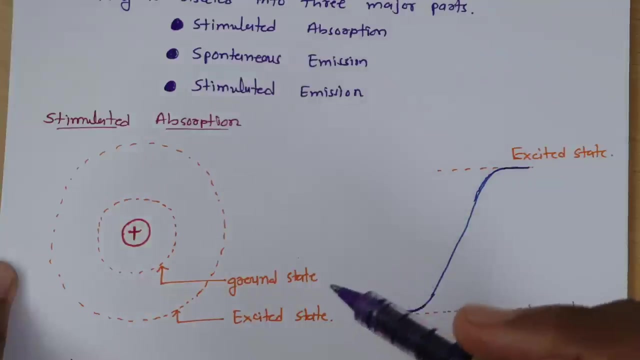 laser working. that i have bisected into three major parts, and fourth part is population inversion. that even i'll explain. so see here to understand working stimulated absorption that is happening, and for that we need to understand quantum mechanics. so quantum physics, quantum physics, mechanics that i'll be explaining. 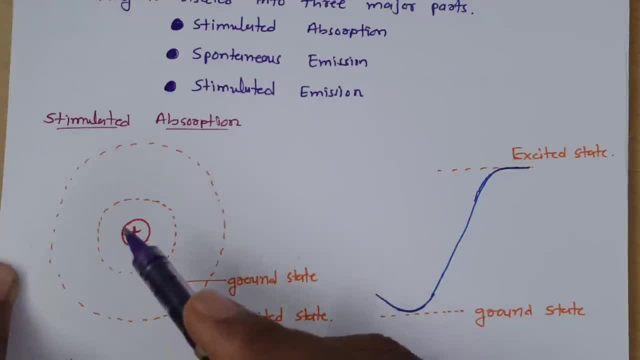 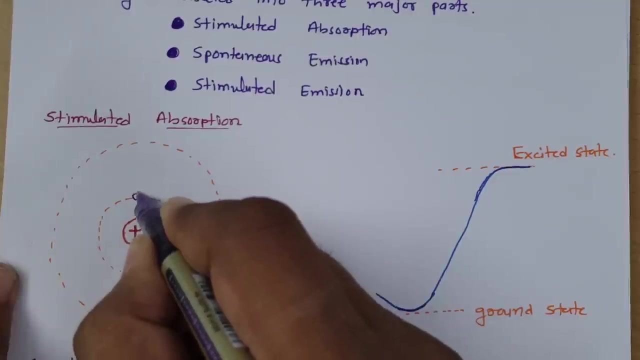 here. now see, if i say we have atom, then at center there will be positive charge, protons and electrons will be there in orbits. so that is what we already know. and usually electron will try to stay with its minimum energy, so it will stay in ground state. so if i say electron is 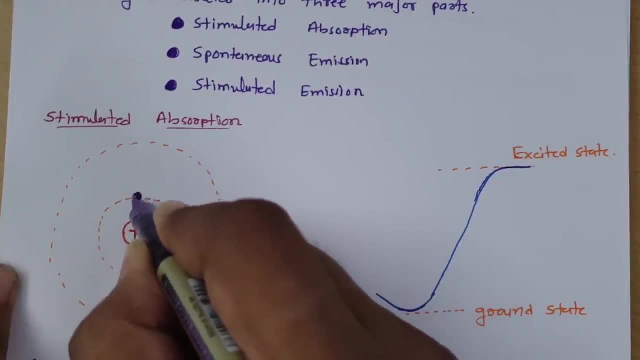 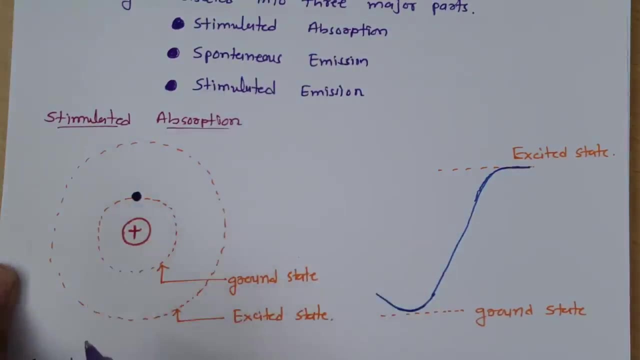 there in ground state over here. so whenever electron that is there in ground state, it will be stable electron. now, what is stimulated absorption? so when electron is there with ground state, here even i'll be showing it with energy diagram. see, this is what energy diagram. so here electron is there in ground state right now, now when we fall light on it. 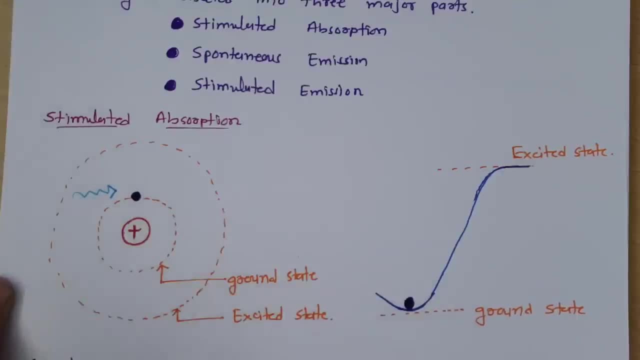 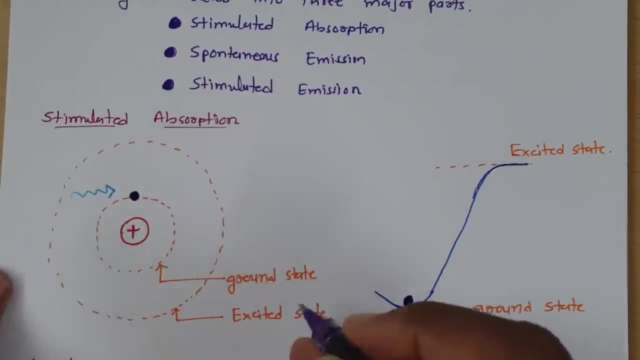 light means photon energy, that we are sending it on this electron. so what happens is this electron that will absorb this energy and it will get excited to higher state of energy. so, for example, right now, if i say with ground state, energy is one unit, one unit energy. 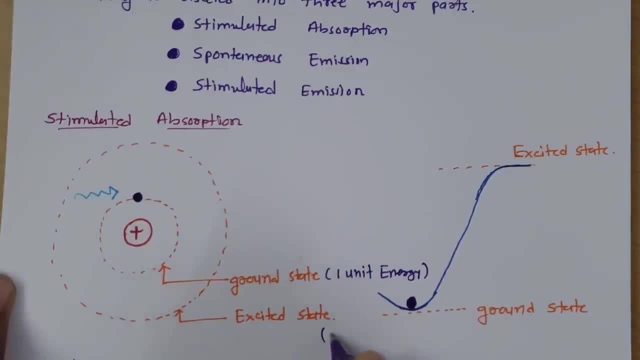 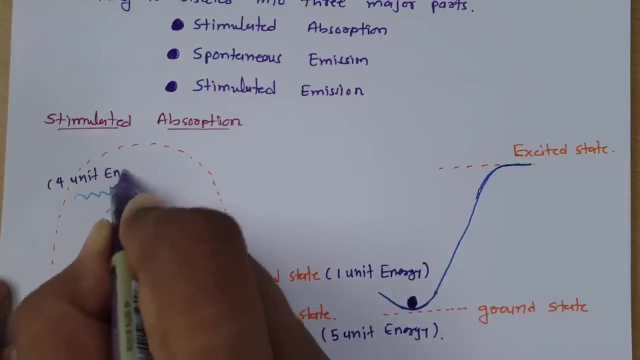 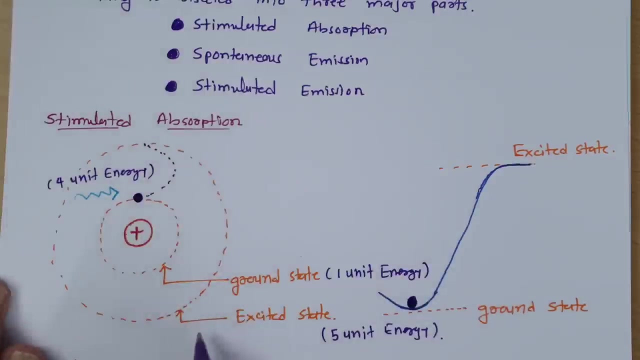 and with this excited state, if i say ilit div wi be discussed by this free unit energy, then by this light, if i give 4 unit of energy, then this electron that will jump from this ground state to excited state. so this electron will come over here, so this electron that will move. 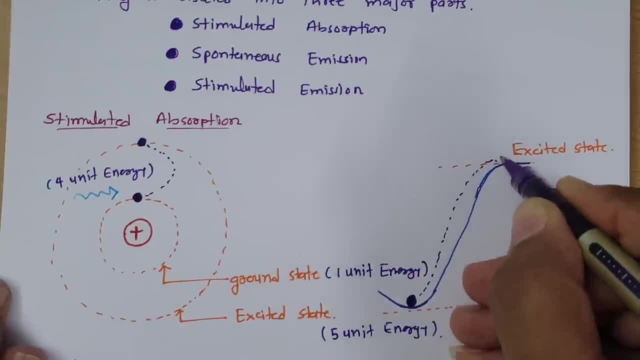 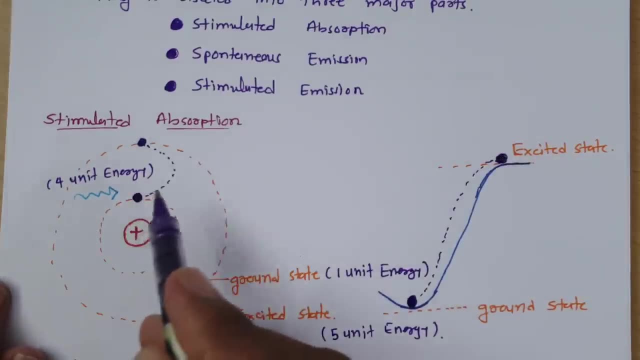 from ground constant state to exited stateigh, from excite state. so electron will connect here, ground state to excited state over here. so this, this is what stimulated absorption, stimulated means by this photon energy. we apply that energy to ground state electron and we energize it, and by energizing it we can move this electron from excited state, from ground state to excited. 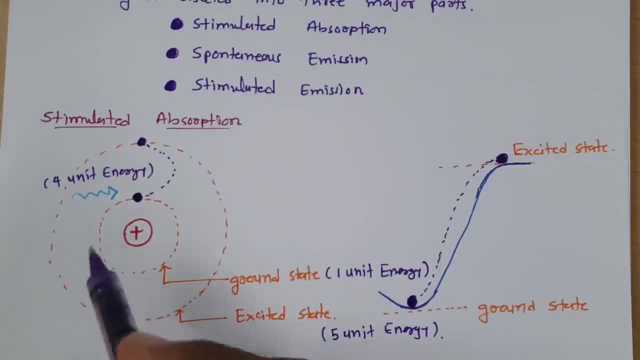 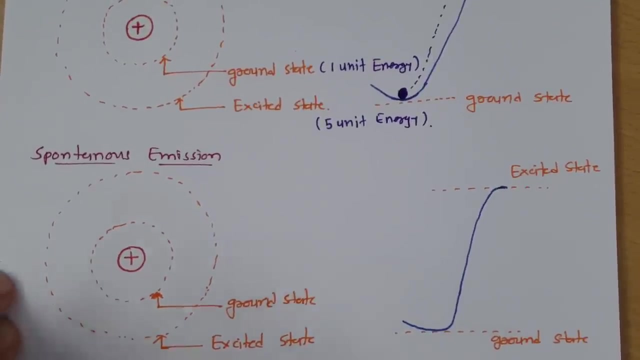 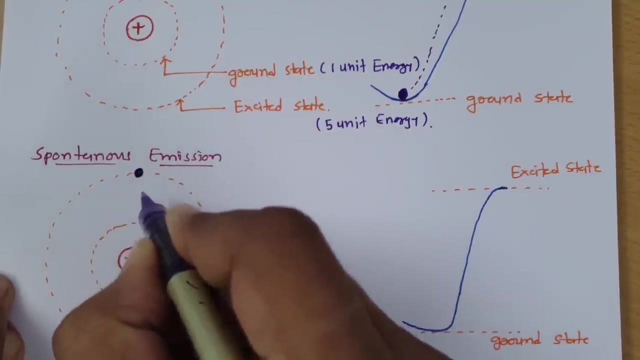 state. so this is what stimulated absorption. so basically, stimulated absorption is to transfer electrons of ground state to excited state by supplying energy using photon energy. now second part is what is spontaneous emission? so spontaneous emission means whenever electrons are there on excited state state and those electrons can move on to excited state as per stimulated 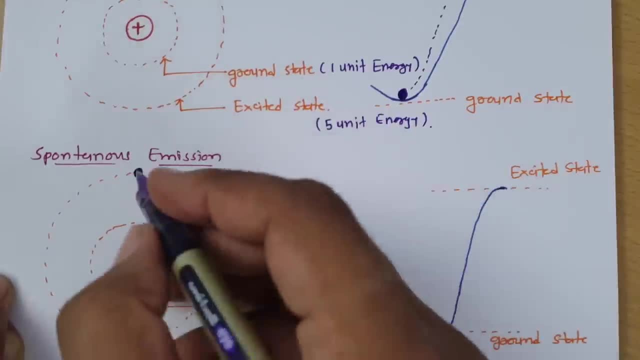 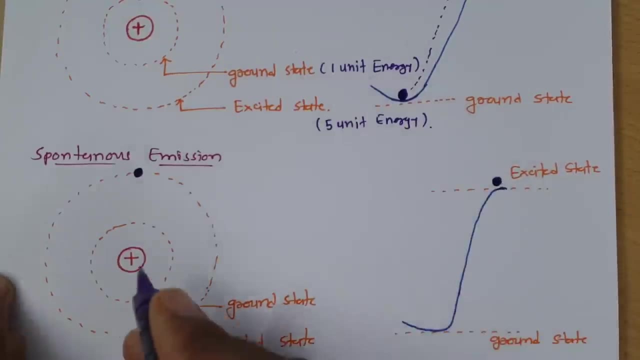 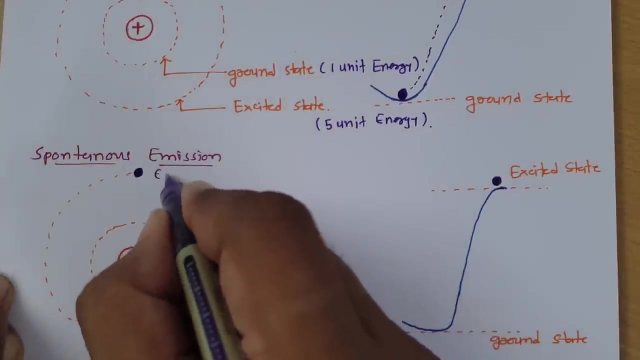 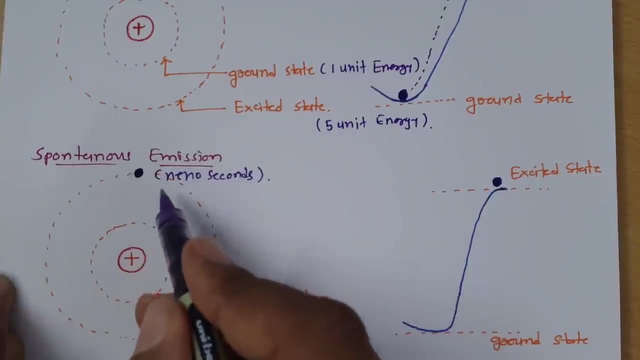 absorption, which i have already explained. so if electron is there in excited state, so here electron is there in excited state. now see life span of electron in excited state. that is there in terms of nanosecond. so those electrons on excited state, that is there in terms of nanosecond and if very 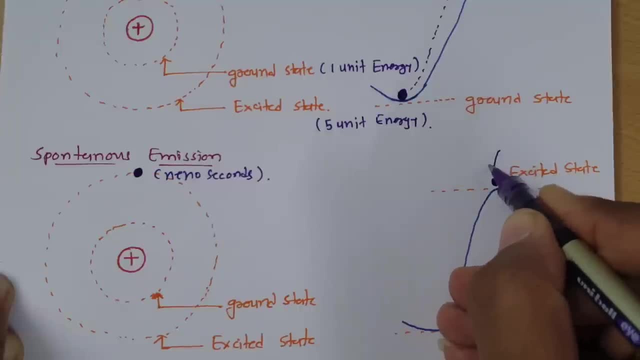 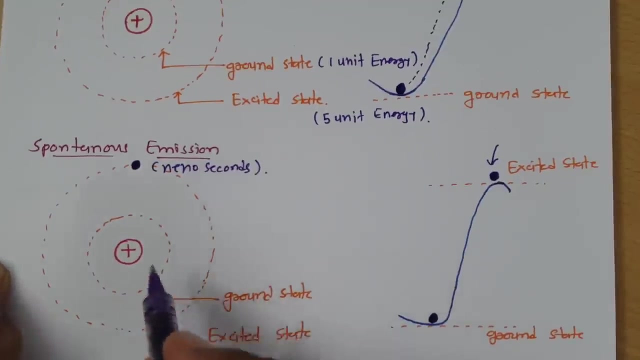 small amount of force. if very small amount of force is happening on this electron, then this electron that will fall back to ground again. that will fall back to ground again. so what happens is, as I have, I have considered, like ground state is having one unit energy and excited state that is having five unit. 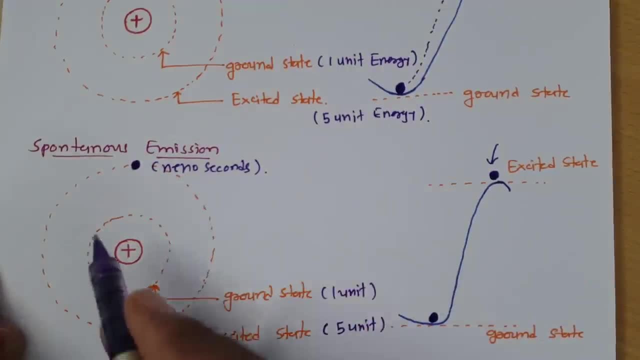 energy. so when this electron, which is there in excited state, when it falls to the ground state, it will release energy. it will release energy and that release of energy that will be there in terms of photons. so this released in energy that is there in terms of photons. so this is what spontaneous emission, so that spontaneous 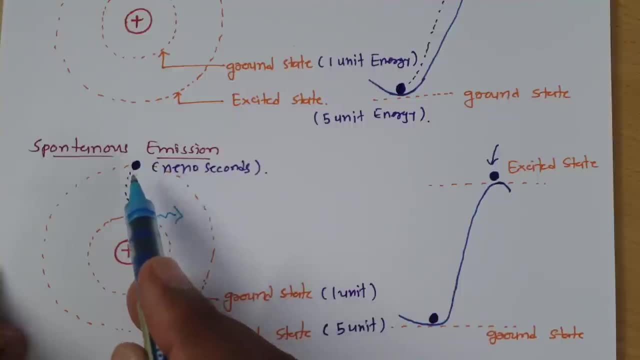 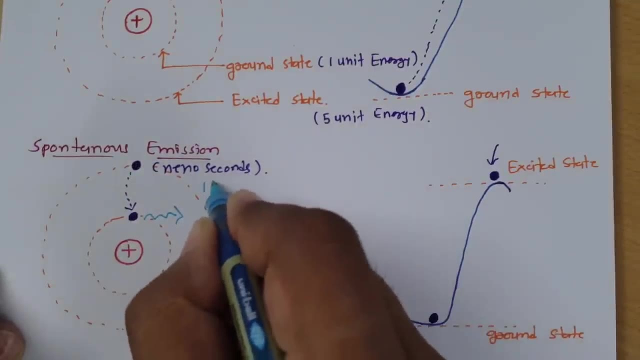 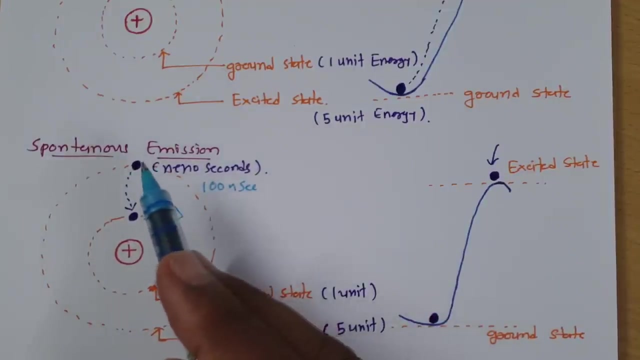 emission. that is happening because of this excited state electrons that is having life span in terms of nanosecond. it is there in terms of hundred nanosecond, so because of life span of the electron's is very less by very small amount of source. this electron. 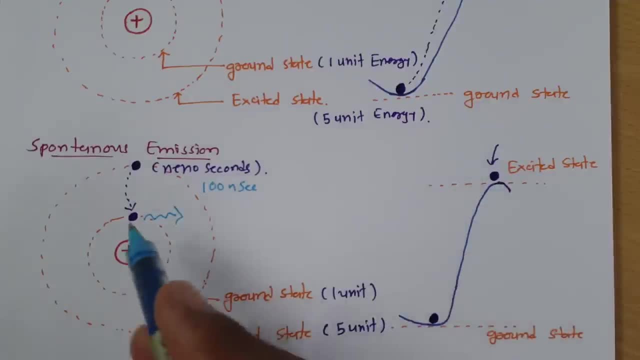 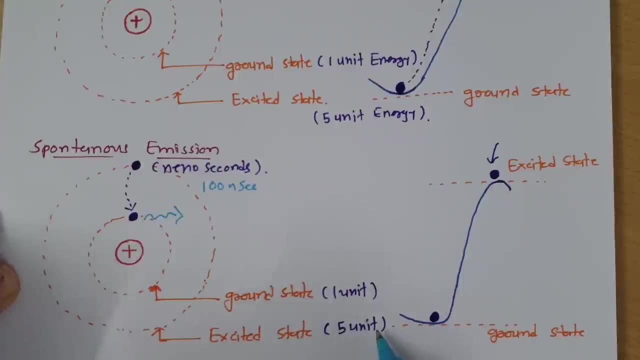 again, will come back to ground state again, and when it comes back to ground state from excited state, excited state is having five unit energy. always it will be having higher energy than ground state. so here this electron will release energy as light, or one can say as photon, and 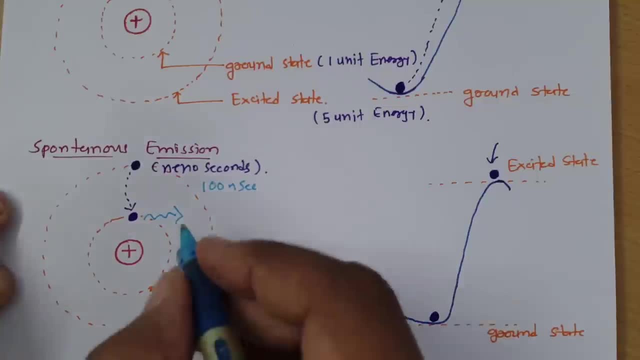 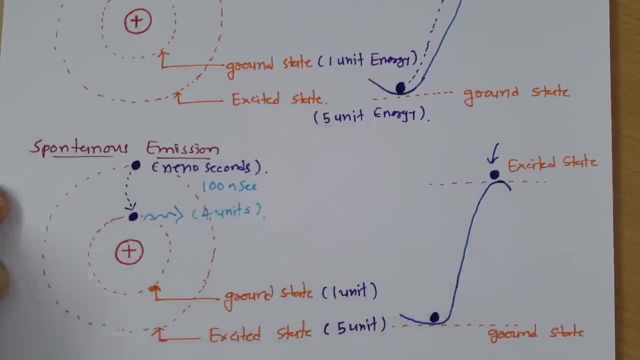 that energy will be 5 minus 1, 4 units. So this is what spontaneous emission. Spontaneous emission means we do not apply any manipulated force to move that excited electron into ground state. So that is what spontaneous emission. Now, what is stimulated emission? So in case of stimulated 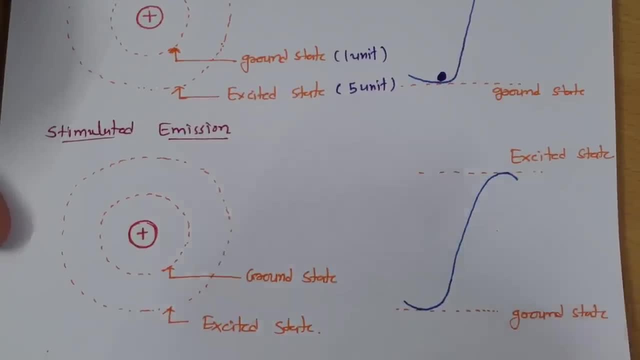 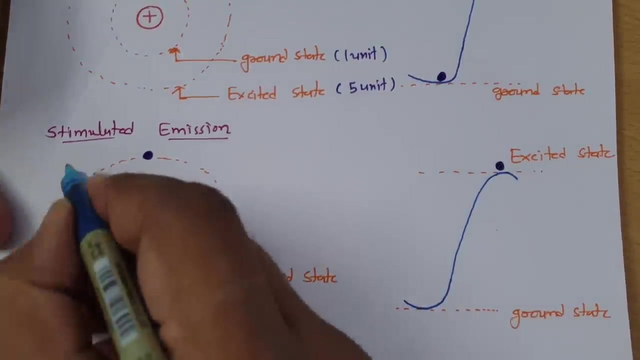 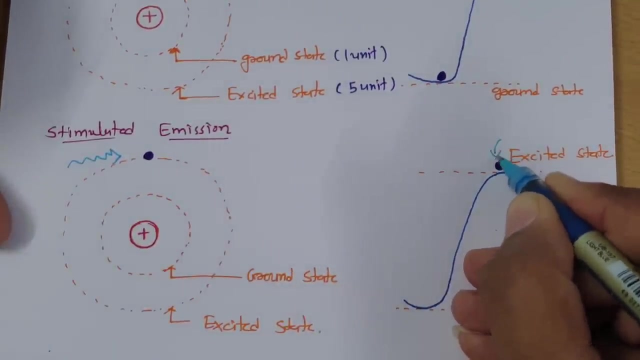 emission. again, if I consider we have electron which is there in excited state, and over here we have electron that is there in excited state, Now all we do is we apply photon energy on it, So as force is applied on it and that force is a force which we have defined it. 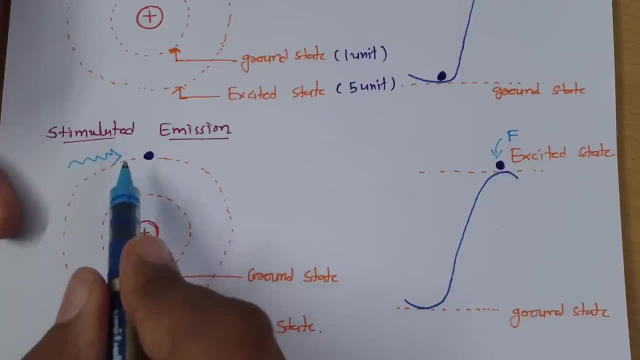 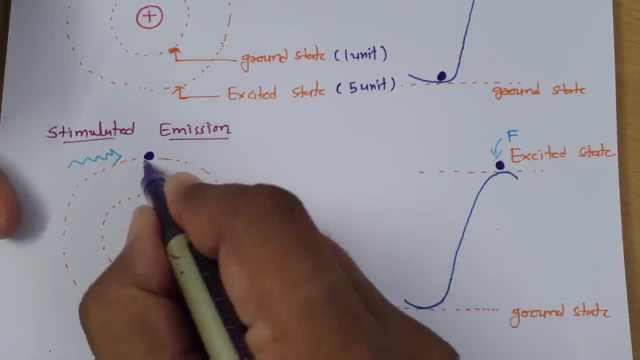 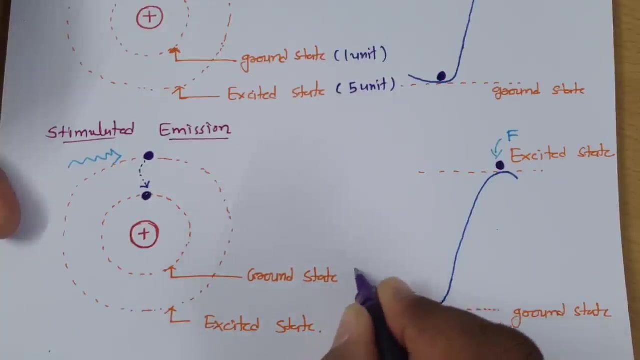 So this is what photon energy that again is falling on to this electron and because of that force now electron is jumping from excited state to ground state and if I consider ground state is having 1 unit energy and excited state is having 5 unit energy, then total after striking this photon 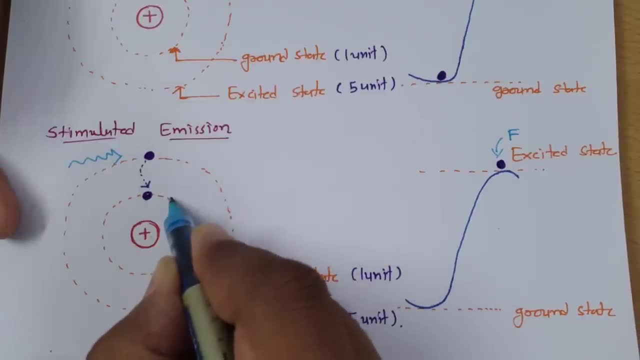 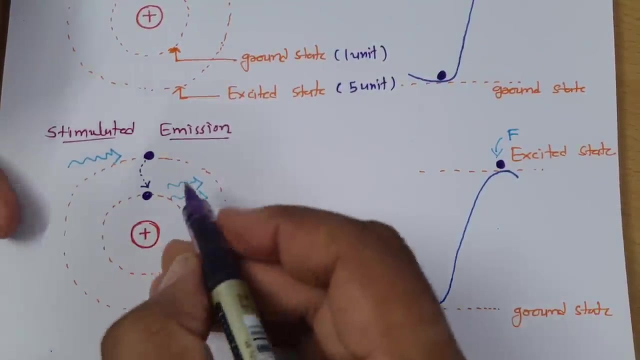 energy on this electron is going to be 5 units. So this is what photon energy is. So this is this electron even will release energy and the energy that was actually striking over here that will not get absorbed, So that energy even will be there. So this is what stimulated emission. So if I say 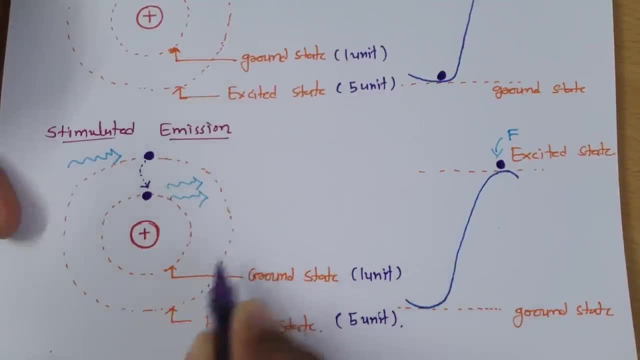 this electron is releasing some energy, then that energy has to be 4 unit over here. So now, if again further there is one another atom that is even getting this energy on it, then that even will release that energy. So this energy will get multiplied and you will be finding, because of 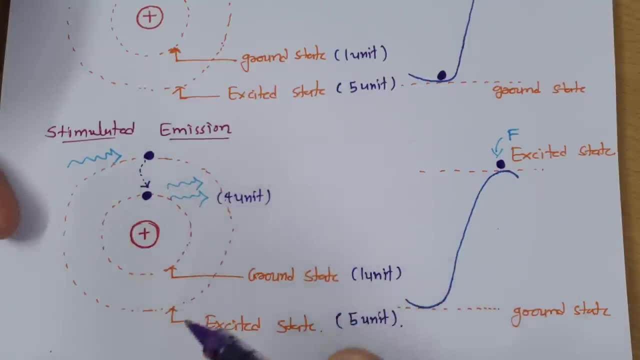 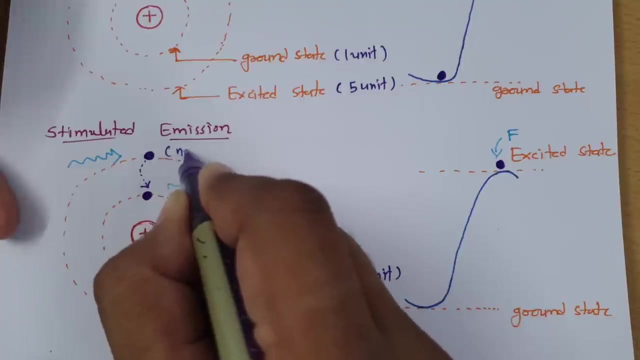 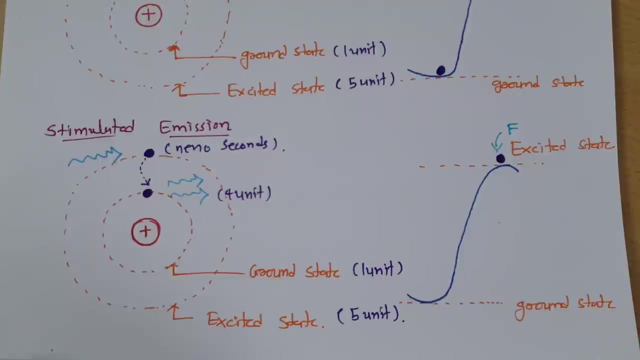 stimulated emission, larger amount of photons can release energy at the same time. But here problem is we have excited state and that is having lifespan of lifespan that is there in terms of nano-seconds. So it is very difficult to have stimulated emission if lifespan of 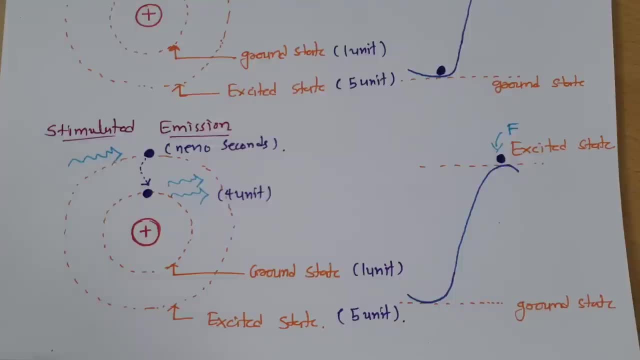 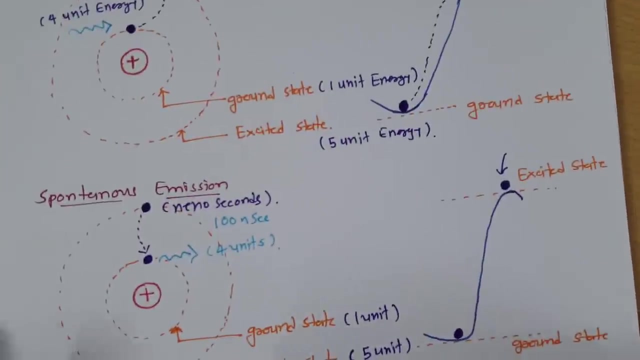 those electrons in excited state is there in term of nano seconds, So in stimulated emission, what we can further add so that we can have more stimulated emission of electrons with coherence emission, So for that terminology which we need to understand, and that is, and that is population. 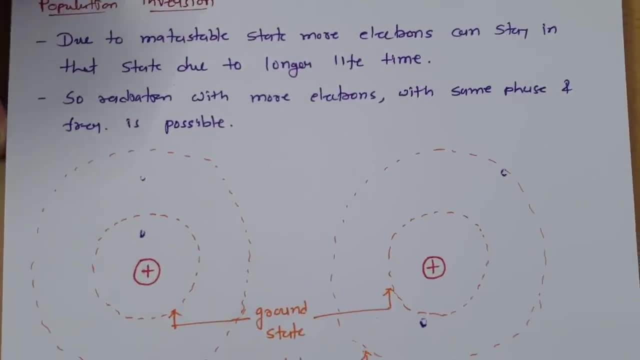 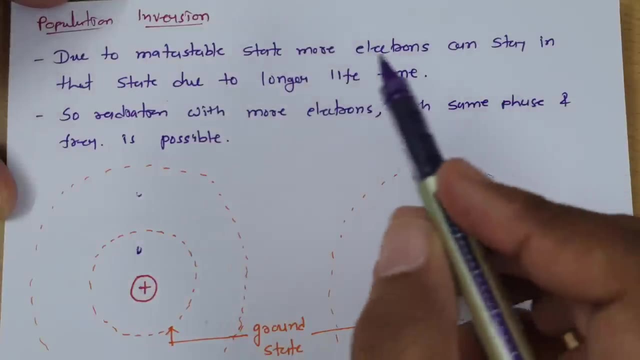 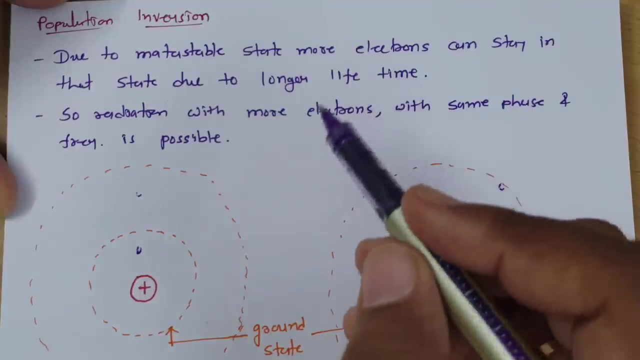 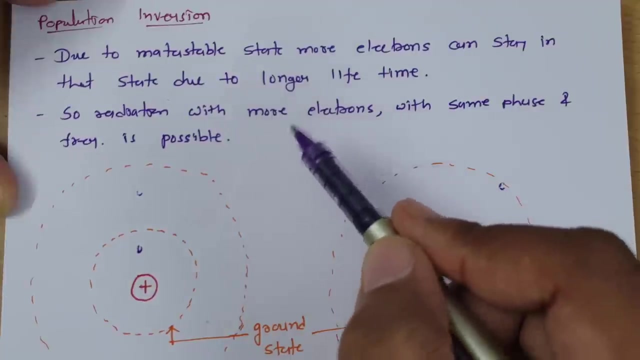 inversion. so now I'll explain population inversion. now see, in population inversion we are adding metastable state with material, so that metastable state that can hold electron for more time as excited state that is having life span in terms of nanosecond. metastable state that is having life span in terms of. 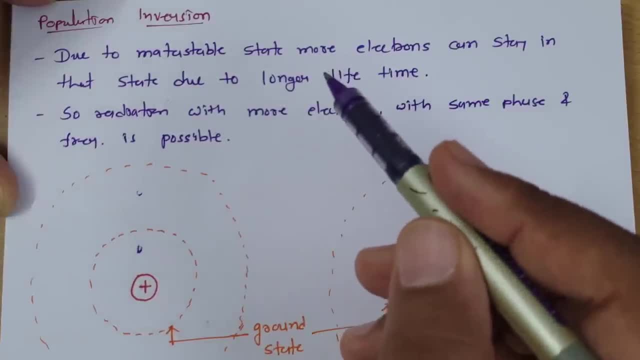 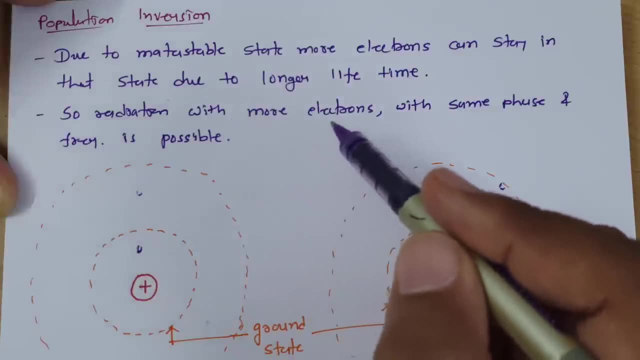 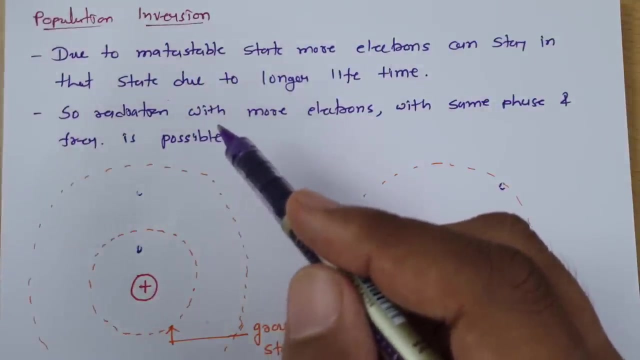 millisecond, so those electrons can stay bit longer in metastable state, so that more electrons can radiate it at the same time with same phase and same frequency. so here we are holding more electrons in in metastable state to have release of energy in same phase, and that is what 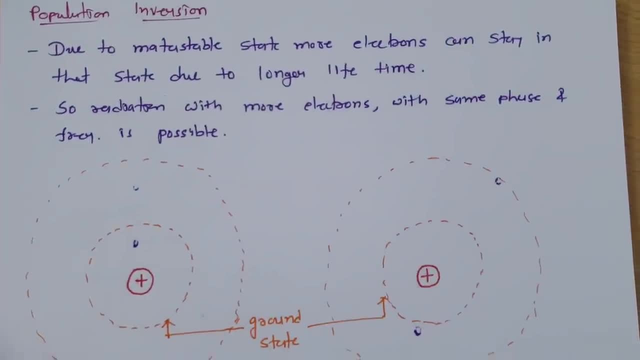 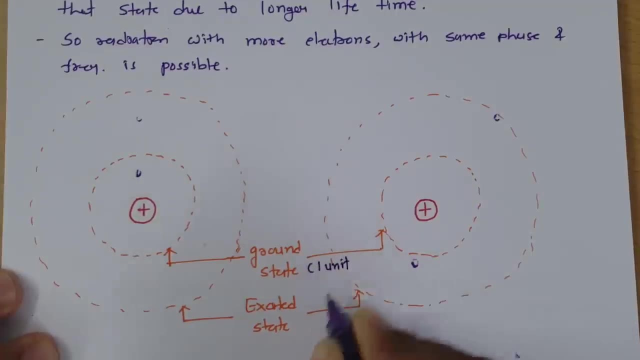 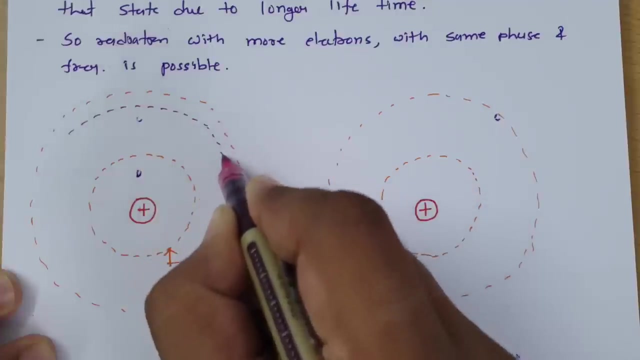 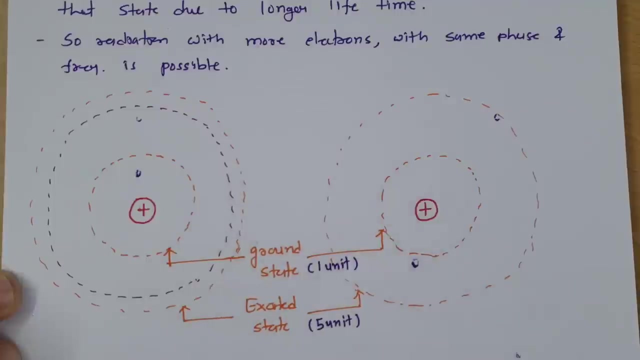 population inversion. so ultimately, here we need to understand metastable state. now see here: if I say ground state is having one unit energy and excited state is having five unit energy, then here we are adding one more energy state that is metastable state. so when you have this metastable state, 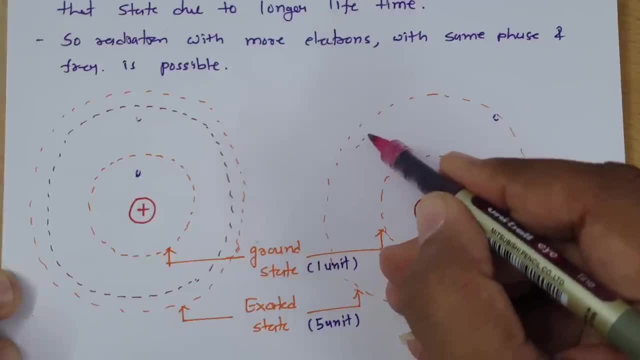 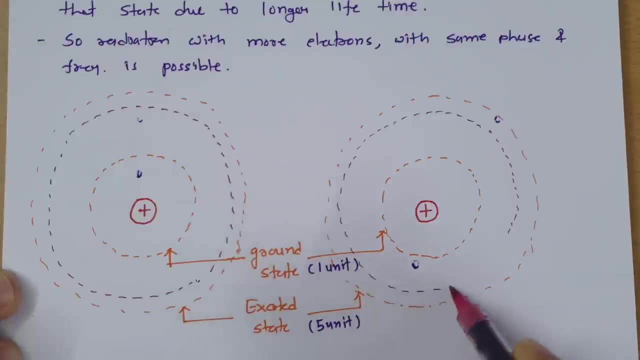 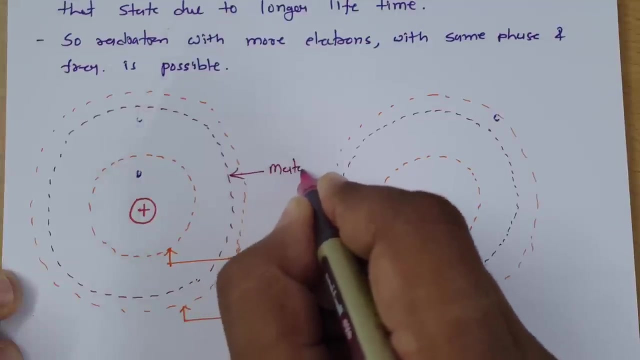 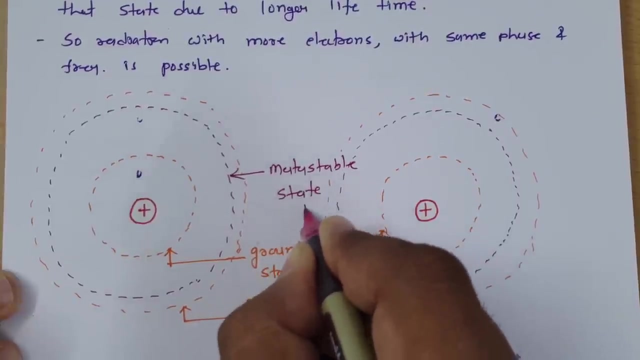 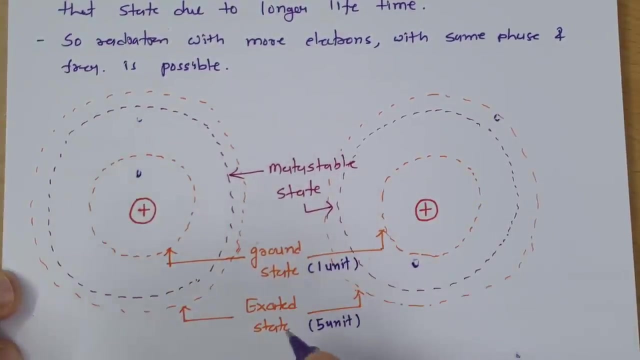 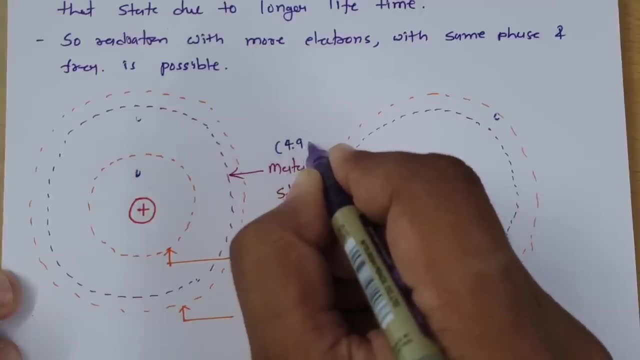 and with this metastable state, energy will be little lower than this excited. and with this metastable state, energy will be little lower than this excited state. if I say energy is 4.9 unit in that case state if I say energy is 4.9 unit, in that case. 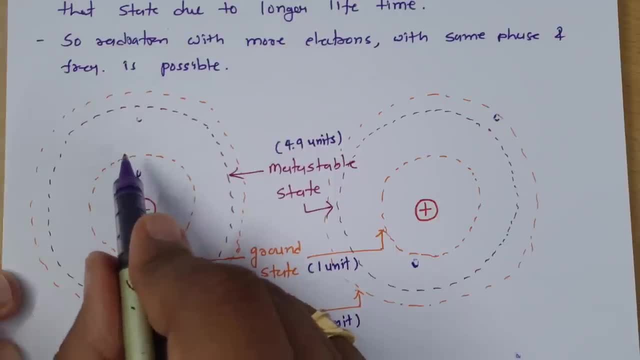 state. if I say energy is 4.9 unit. in that case, what happens is like when electron. what happens is like when electron. what happens is like when electron is there in ground state and when we excite is there in ground state and when we excite. 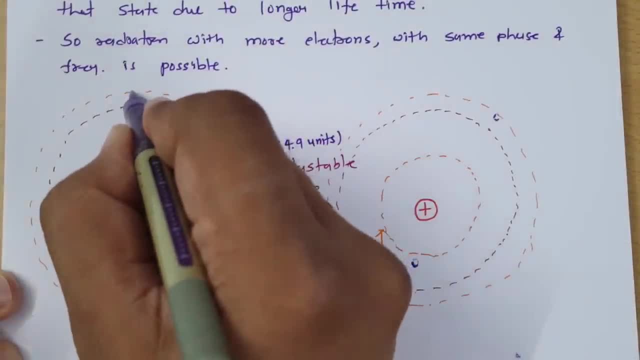 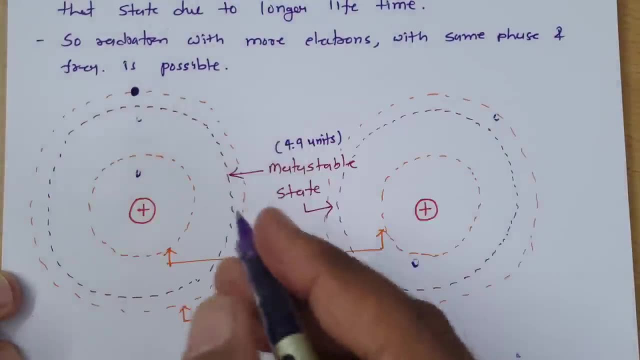 is there in ground state and when we excite that by applying energy, that, by applying energy that, by applying energy electrons over here, that will move to excited electrons over here. that will move to excited electrons over here. that will move to excited state. but, as I have told, excited. 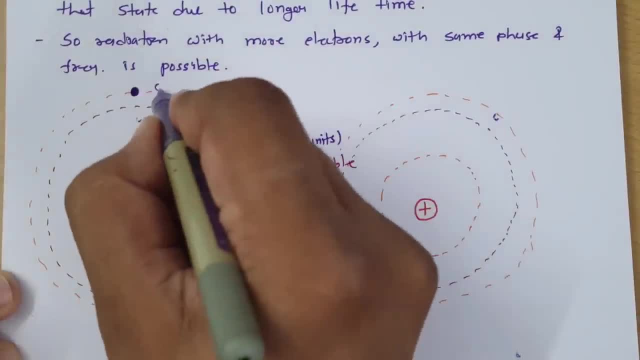 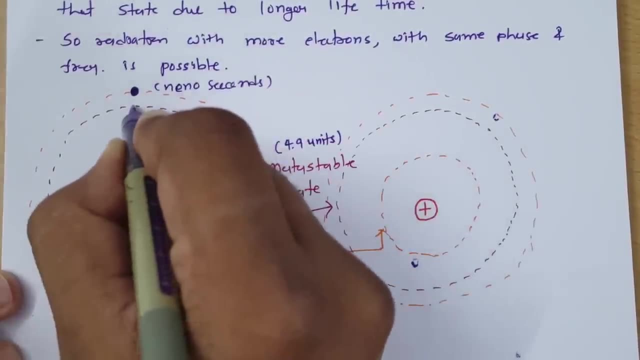 state but, as I have told, excited state. but, as I have told, excited state can hold electrons with lifespan in state. can hold electrons with lifespan in state. can hold electrons with lifespan in terms of nanoseconds, but lifespan of metastable state that. but lifespan of metastable state that. 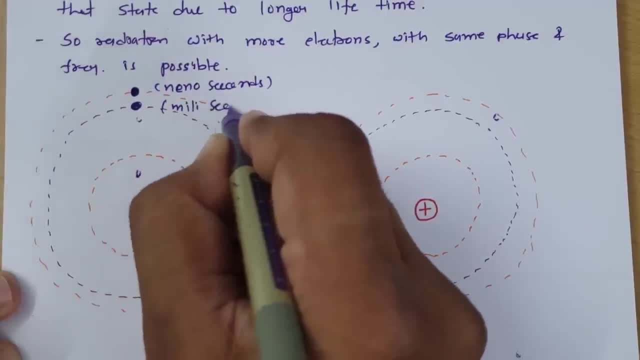 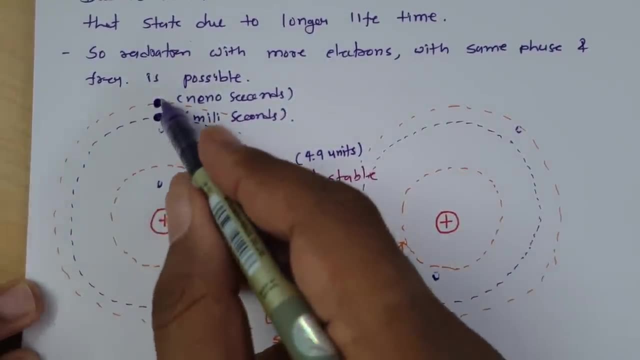 but lifespan of metastable state, that is there in terms of millisecond, so as is there in terms of millisecond, so as is there in terms of millisecond, so as life span of metastable state is more, life span of metastable state is more, life span of metastable state is more these electrons, which is there in 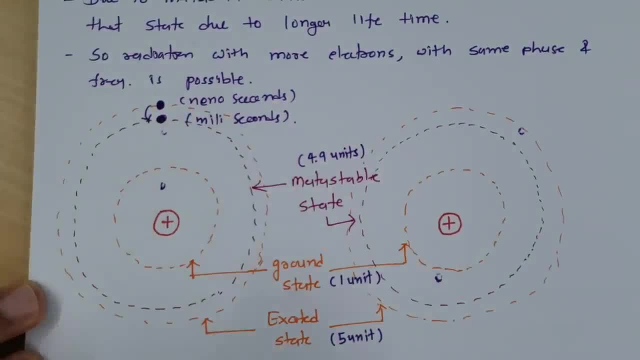 these electrons, which is there in these electrons, which is there in excited state, that will move into excited state, that will move into excited state, that will move into metastable states. so we'll be finding metastable states. so we'll be finding metastable states. so we'll be finding more electrons. that is staying in. 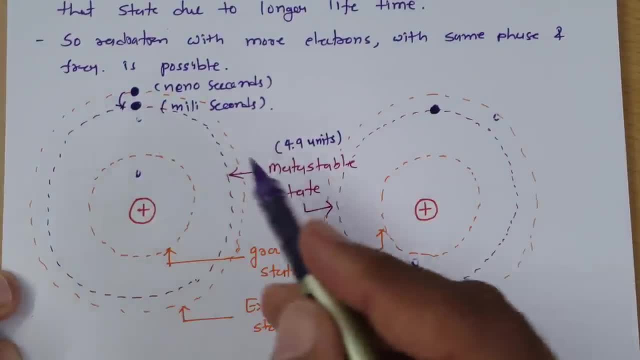 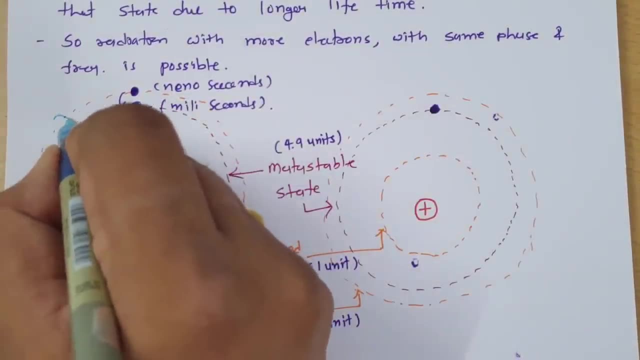 more electrons. that is staying in more electrons. that is staying in metastable state, as it can hold metastable state, as it can hold metastable state, as it can hold electrons for longer life span. now see electrons for longer life span. now see electrons for longer life span. now see as if we apply photon energy- this 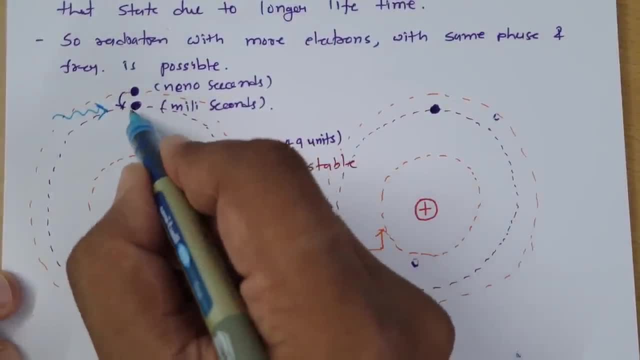 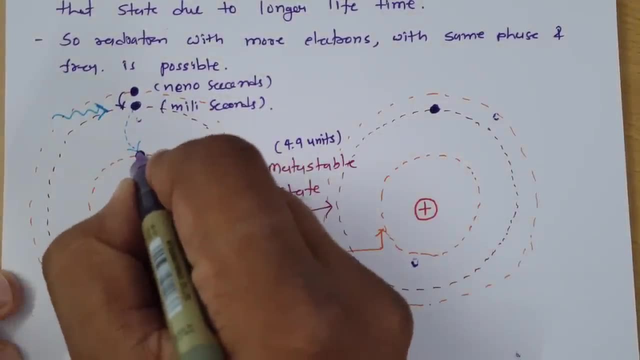 as if we apply photon energy, this, as if we apply photon energy, this electron electron that will jump from higher energy state to that, will jump from higher energy state to that, will jump from higher energy state to ground state and as it is actually moving from higher and as it is actually moving from higher, 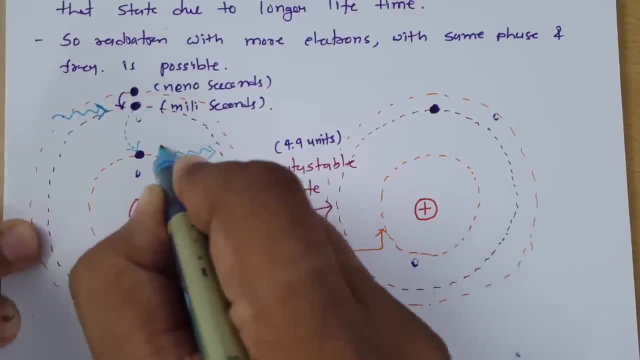 and, as it is actually moving from higher energy state to ground state, it will energy state to ground state, it will energy state to ground state, it will release energy and those energy will be release energy and those energy will be release energy and those energy will be in phase. and now this energy, that is. 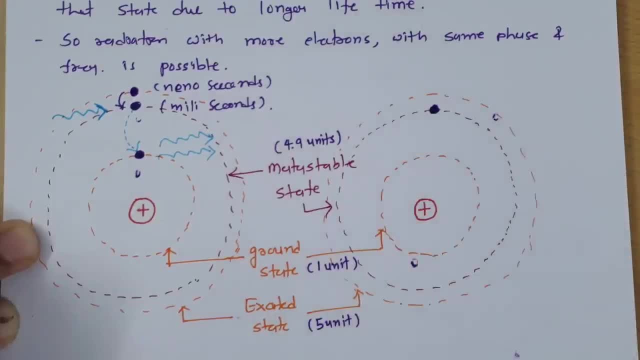 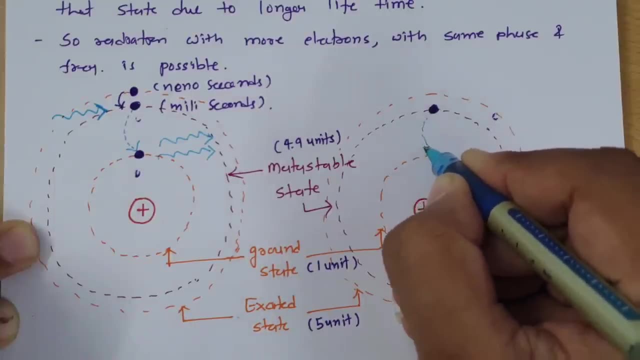 in phase. and now this energy that is in phase, and now this energy that is moving to another atom, and that will moving to another atom, and that will moving to another atom, and that will again, again, again, again move this electron like this, and this electron will again. 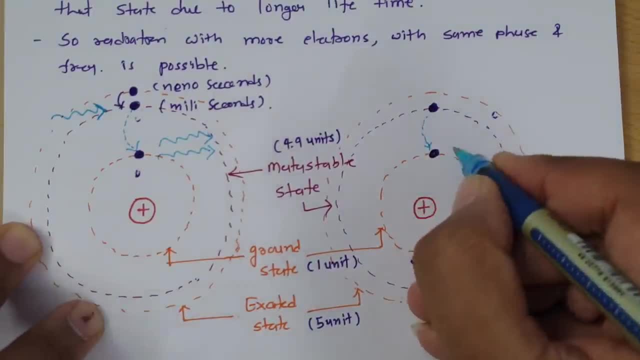 like this and this electron will again like this and this electron will again come back to ground state. so you'll be come back to ground state. so you'll be come back to ground state. so you'll be finding now more energy here to photon, finding now more energy here to photon. 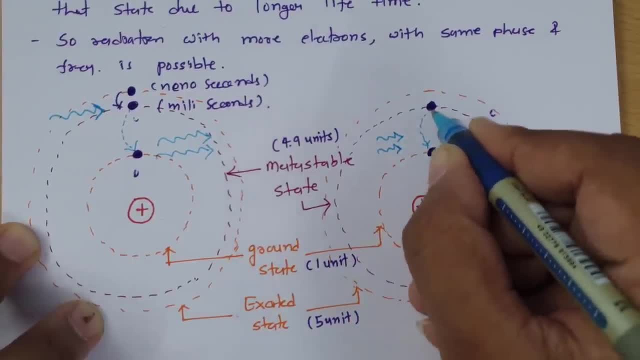 finding now more energy here to photon, energy that is coming, that one can see, energy that is coming, that one can see, energy that is coming, that one can see. and now, after moving this electron from, and now after moving this electron from, and now after moving this electron from metastable state to ground state, you can 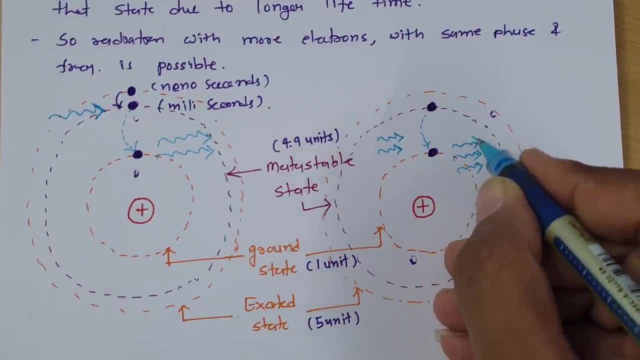 metastable state to ground state. you can metastable state to ground state. you can see coherent energy. see coherent energy, see coherent energy. coherent means same frequency and same phase. coherent means same frequency and same phase. coherent means same frequency and same phase that is getting released. so because 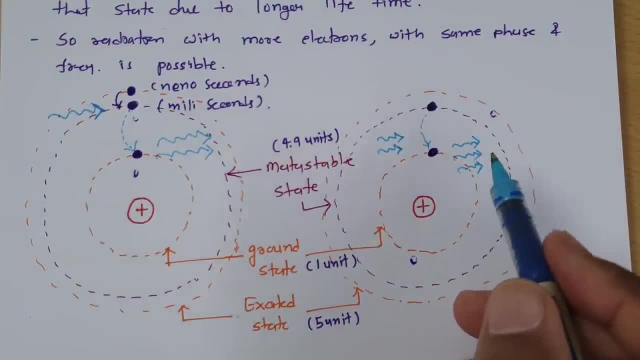 that is getting released. so because that is getting released, so because of population inversion, same phase with. of population inversion, same phase with. of population inversion, same phase, with same frequency and wavelength, we are same frequency and wavelength. we are same frequency and wavelength. we are releasing energy with magnet more. 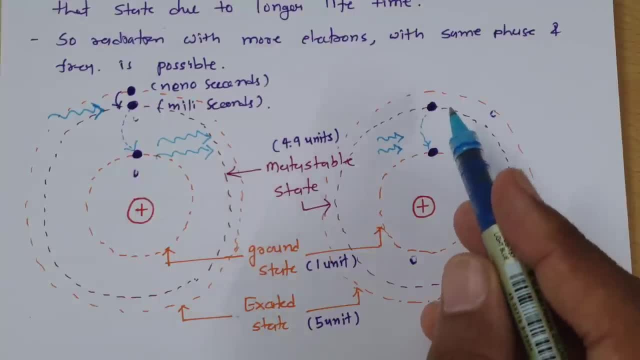 releasing energy with magnet, more releasing energy with magnet, more magnitude of transition from excited magnitude of transition from excited, magnitude of transition from excited state to ground state. so that is what state to ground state, so that is what state to ground state, so that is what population inversion. and here you will. 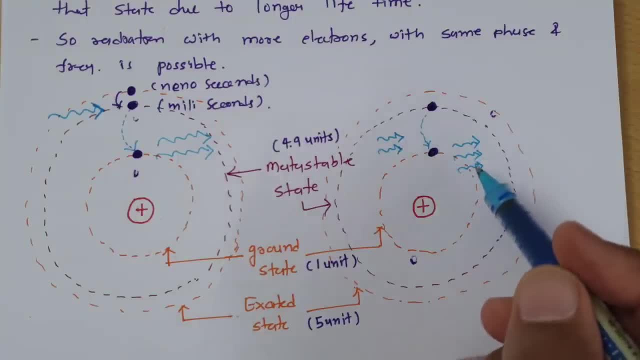 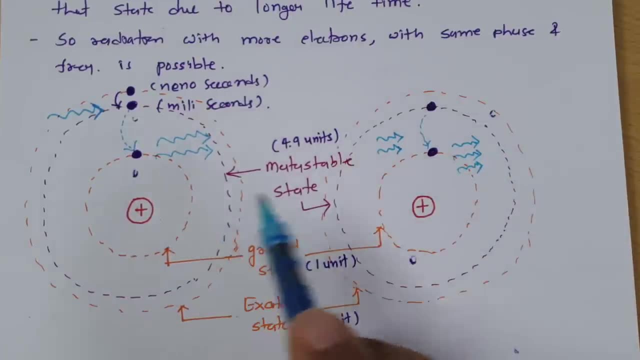 population inversion, and here you will population inversion, and here you will be finding higher amount of energy, of be finding higher amount of energy, of be finding higher amount of energy of radiation. that is happening with coherent and same phase and frequency radiation. So this is how population 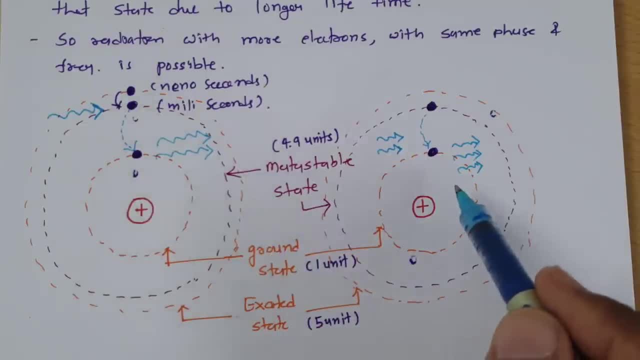 inversion, that is, increasing directivity of radiation of photons, and as if this energy transition from higher energy state to lower energy state is staying in the range of 4000 angstrom to 8000 angstrom, which is visible region- in that case one can see light is getting emitted. 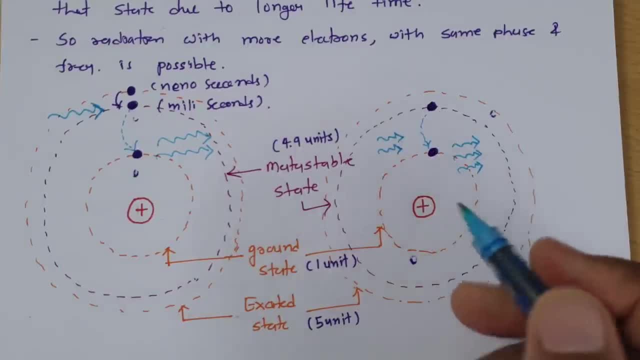 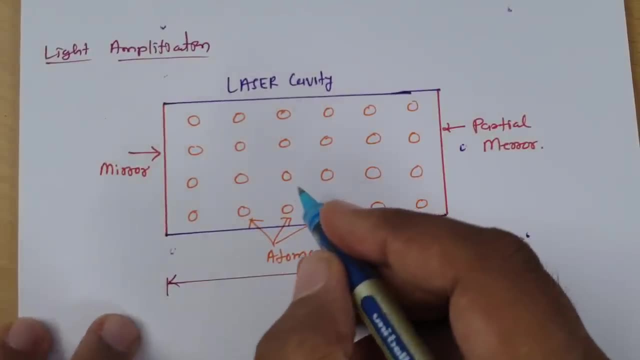 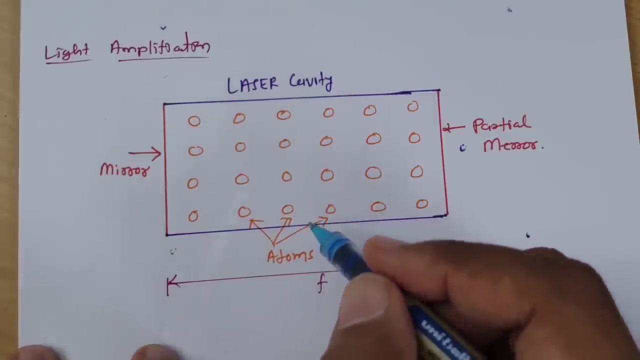 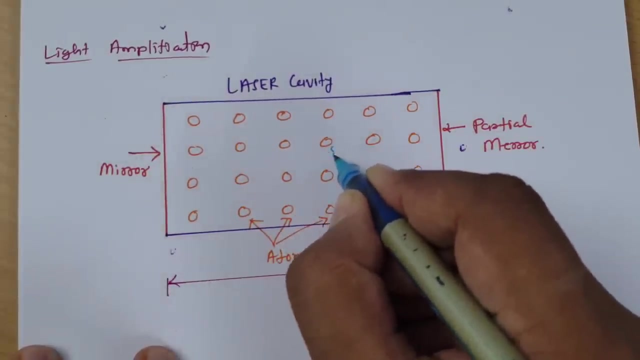 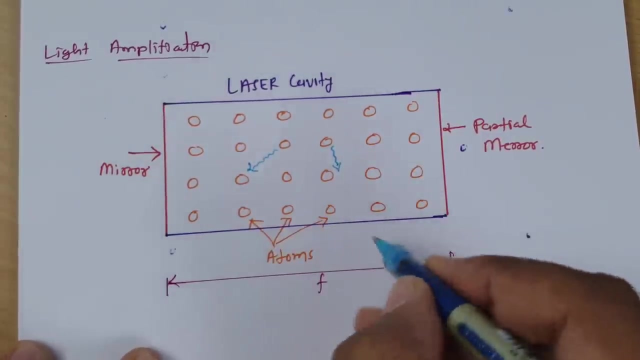 with some finite colors. Now I'll explain you how light amplification is happening. So see, as we have discussed in population inversion, metastable state can hold electrons for more time period. When you add light over here, those electrons will be generating some transition, and few of that transition that I am showing over here. 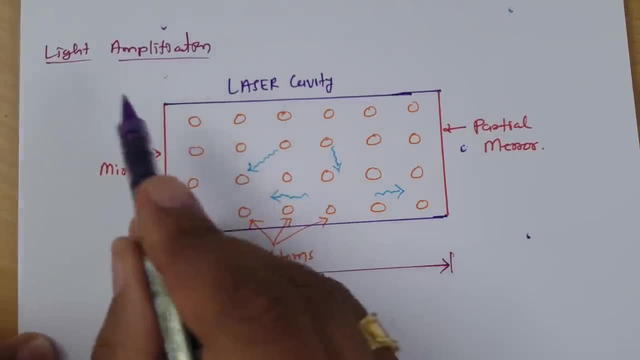 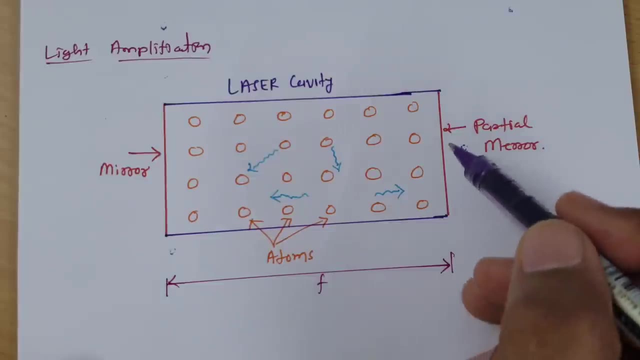 but see, if you see this cavity, then here there is one mirror and here there is partial mirror. so because of mirror is have mirror is there in this two side, other than this two side transition will get cancelled. so this and this transition that will get cancelled, only this two. 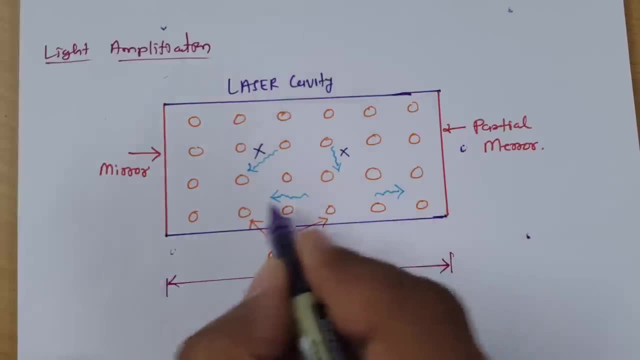 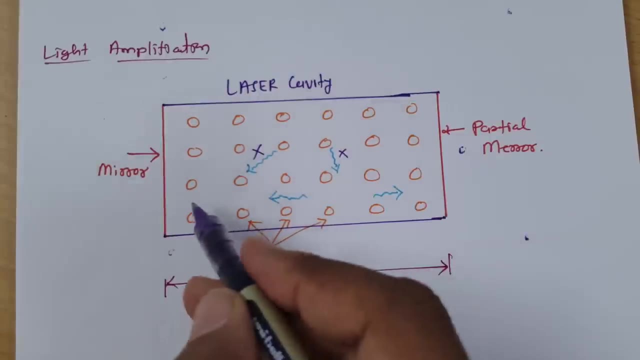 transition of photon energy that will get move in this direction like this, it will actually go in this direction as well, as it will go in this direction and whenever this two signals here I am just showing two signals, so this two signal- that is, having additive phase, at that time signal will increase. and when there is destructive phase, at that time 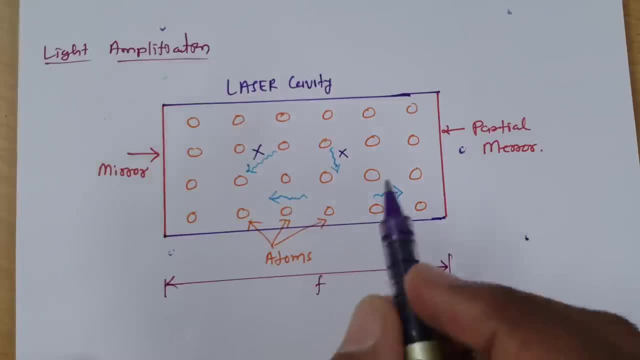 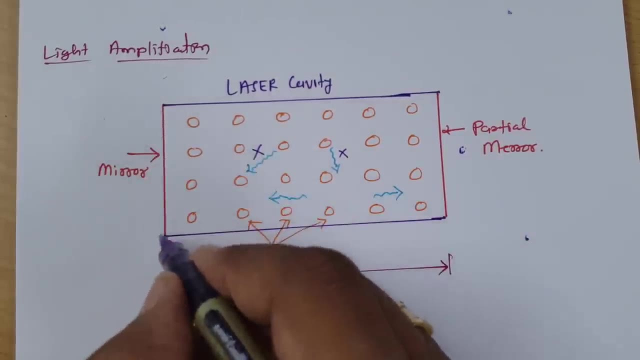 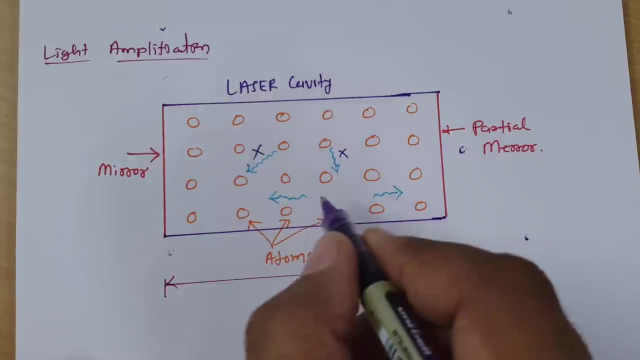 signal will decrease, so it will generate standing pattern. so transition which is happening in the direction of this mirror, where over here there is mirror and over here there is partial mirror, so partially signal will get reflected from this direction to this direction and and completely signal will get reflected from this direction to this direction. multiple signals will